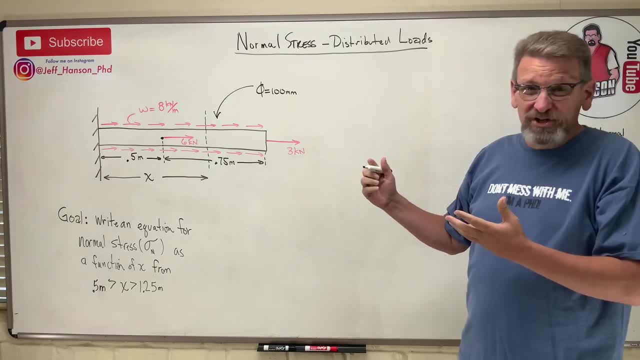 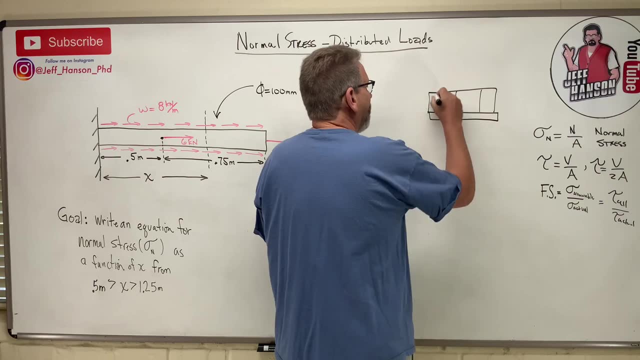 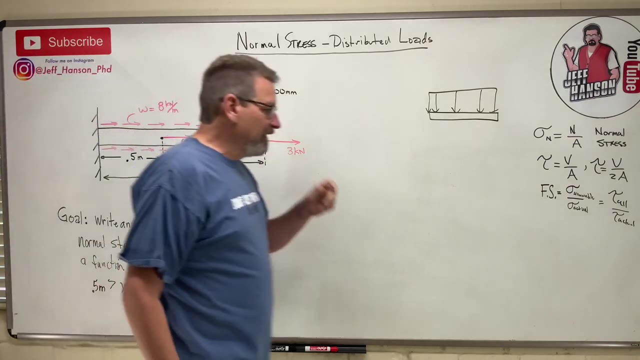 So for this problem, right? we're used to distributed loads from like statics looking like, looking like this, maybe, right? Well, why would you have a load that is along the beam? Well, think about if you had a beam. I have a beam, it's just my little thing here, right? 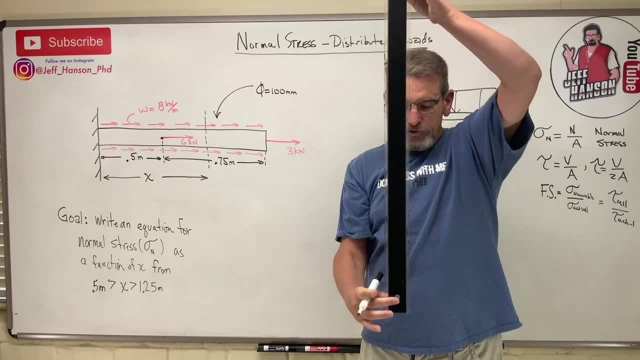 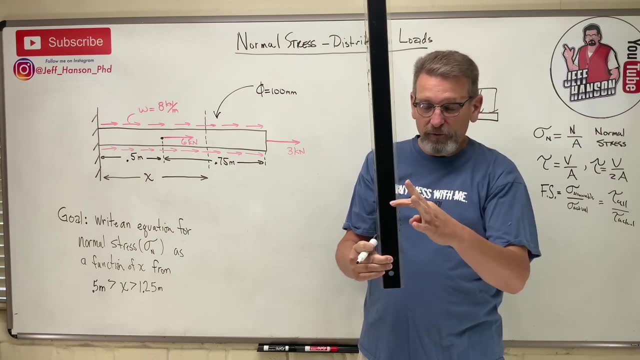 This thing has weight, and so if I measure a point right here, right, if I'm this point right here, I only have this much weight acting on me. If I go this point right here, it's a little farther up now I have a little more weight that's trying to stretch me, right. 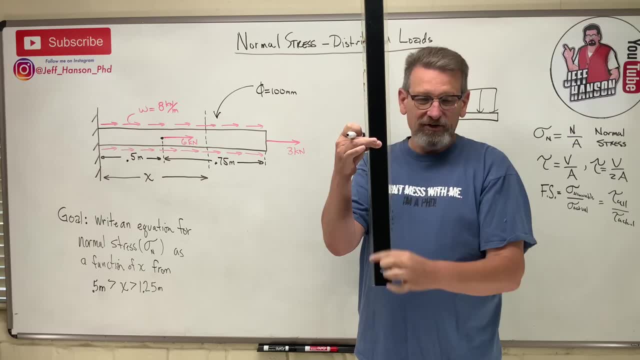 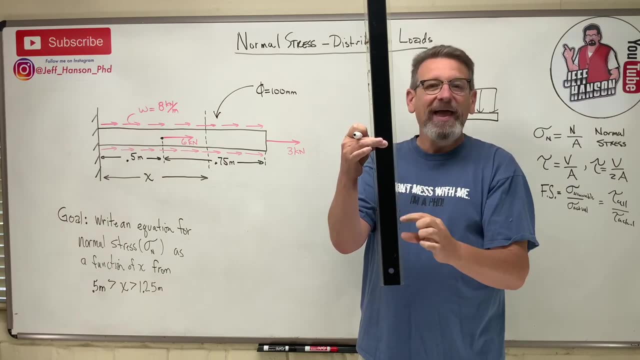 If I look at a point right here, I have even more weight trying to stretch me right. So as I go along here I've got distributed load, this per unit length weight that's being added to the beam and it's the same this way. 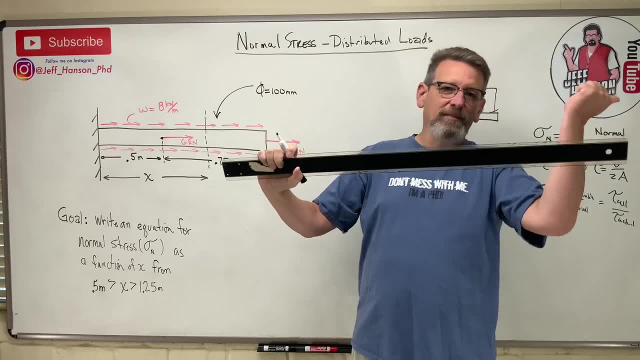 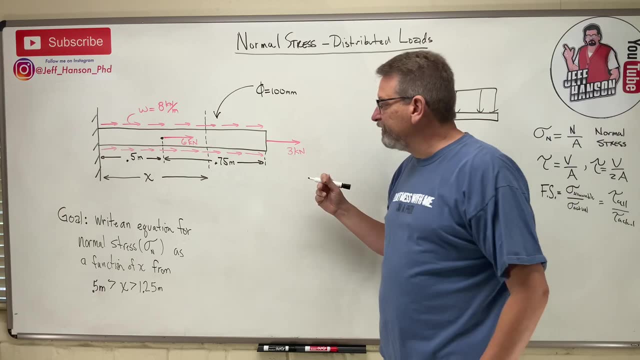 If I do it this way and I say there's a load, a distributed load, pulling that way along the beam, it makes a little bit of a difference. It makes a little more sense when you think about it with gravity. but it could be like this: 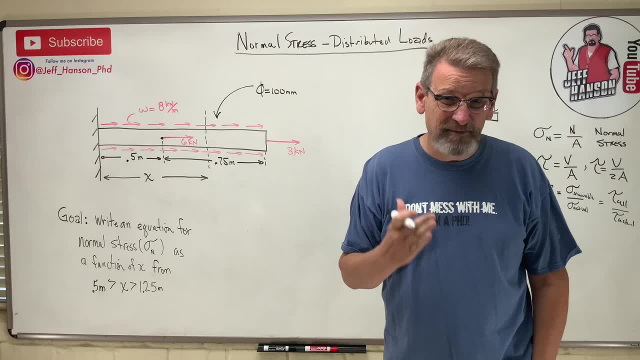 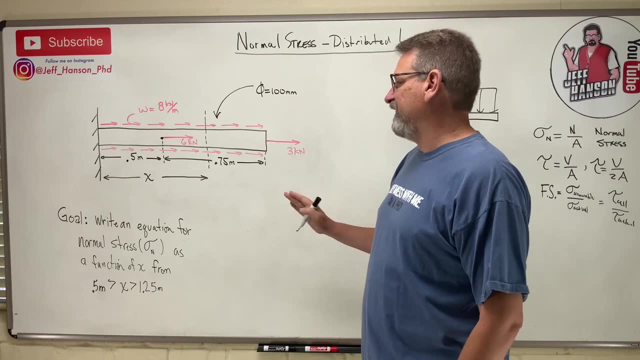 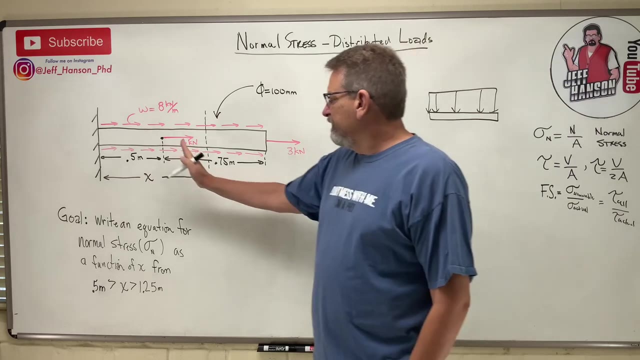 They want us to write an equation for normal stress, sigma stress, that's P over A stress, right, As a function of X. what is X? X is just a distance, okay, from here over to here, from 0.5, which is this point here- to 1.25, which is this point out here. 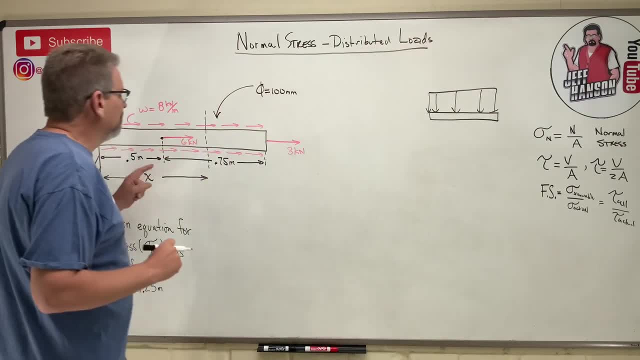 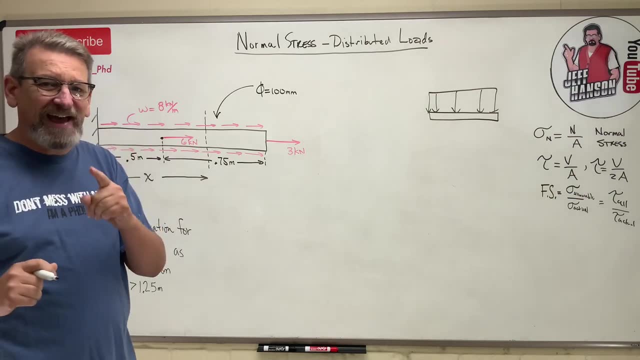 Now here's a question for you. okay, If you're out here somewhere. what is the 6 kilonewtons? what is the 6 kilonewtons acting on? okay, Imagine, this beam is a big rubber band, right? 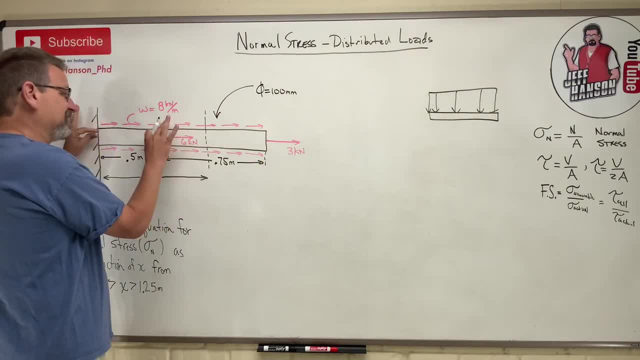 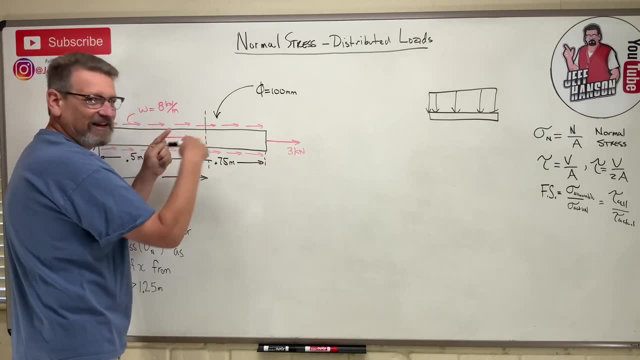 If I grab that rubber band right in the middle, right here at 6, right, and I stretch it with 6 kilonewtons, then what is that 6 kilonewtons doing to this side of the rubber band? 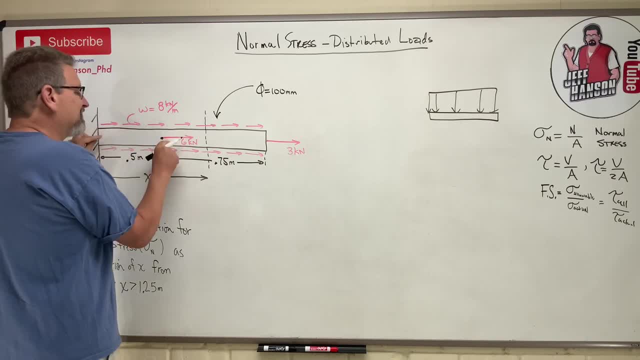 Nothing, It's just along for the ride, right. So the 6 here only affects this, This portion of the beam, whereas the 3, right. if I add the 3 to my rubber band, I've got a weight in the middle. when I add that one, the whole thing stretches. 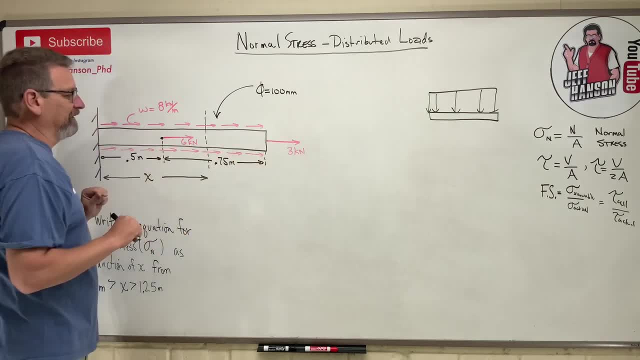 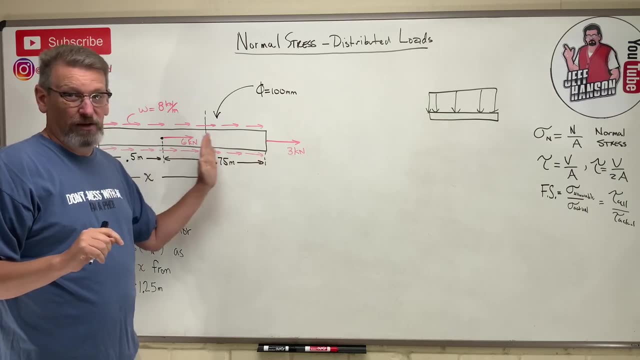 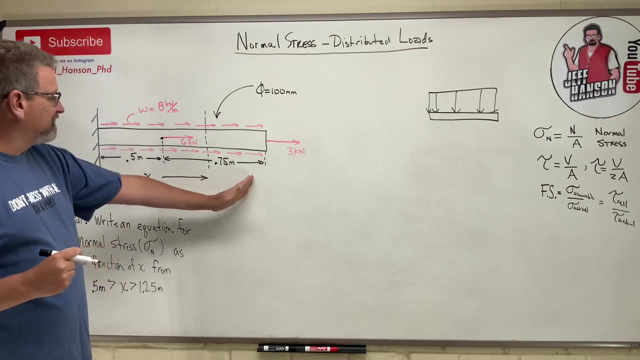 So this guy is going to affect this part of the beam and that part of the beam. Does that make sense? So the 6 actually doesn't affect this part of the beam at all. okay, So how do we do this problem? So they want from 0.5 to 0.75, in other words, anywhere in this range here. 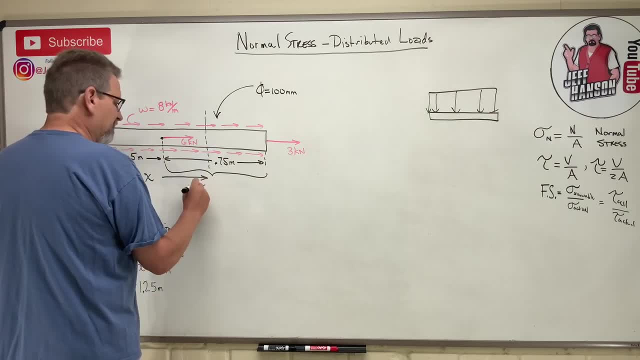 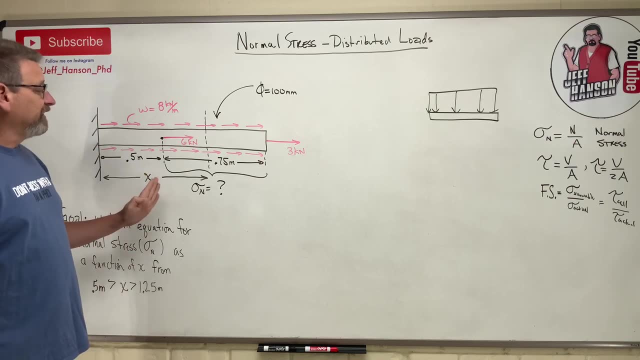 give me an equation: sigma n equals something right for that part of the beam, okay. Well, let's look at it at a distance of x. Where is x? x is just any point right. We're just going to pick a place. wham, right there. 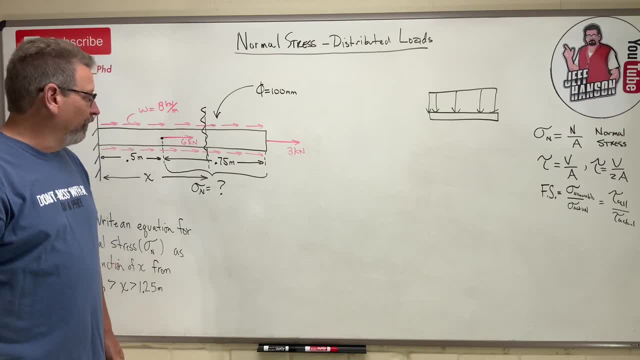 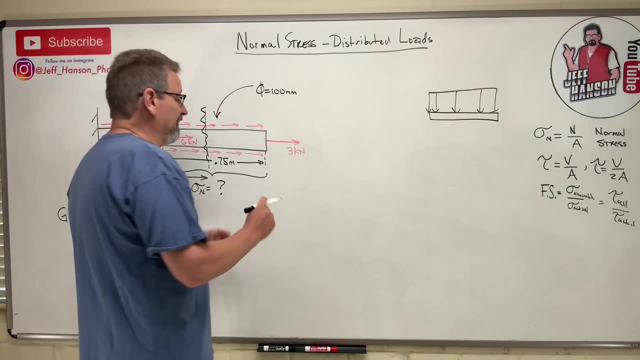 And you can remember this back from statics world, right? What do we do when we cut a beam? You know you have to draw a free body diagram of that side of the beam. Let's draw a free body diagram. That side of the beam look like this: 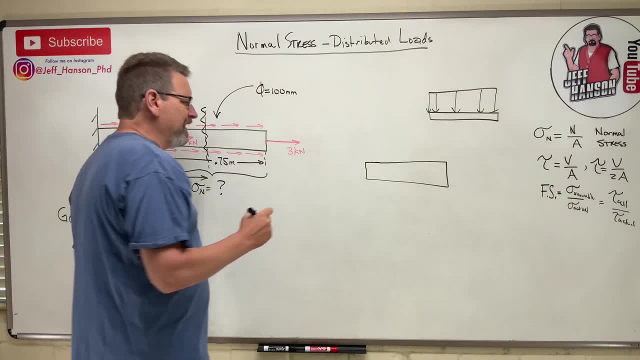 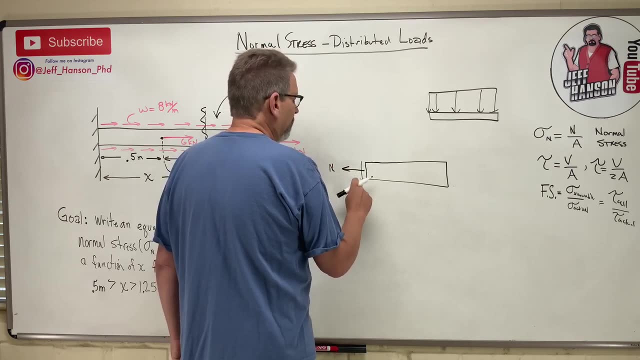 And where we cut that beam, you must have a m and v right, So you'd have: there's the v, there's n. Oh, that's going to be going up, isn't it? on this side, According to the positive sign convention that we all know and love, right? 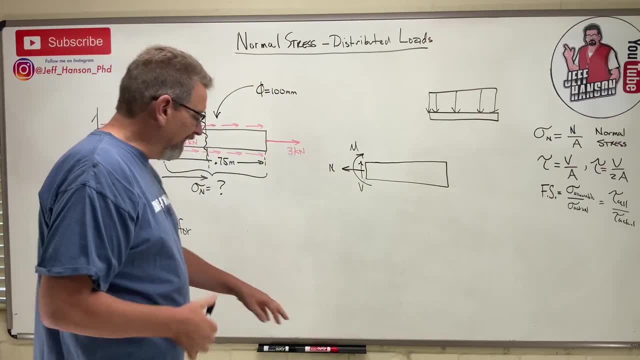 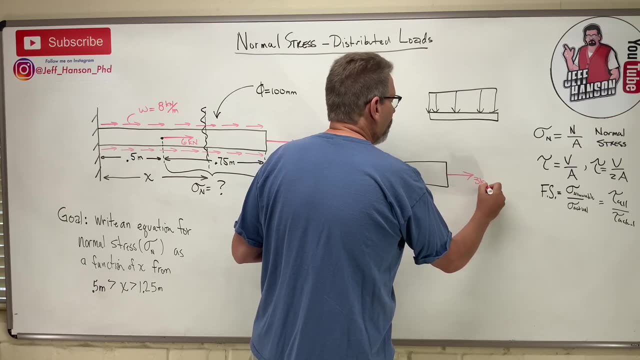 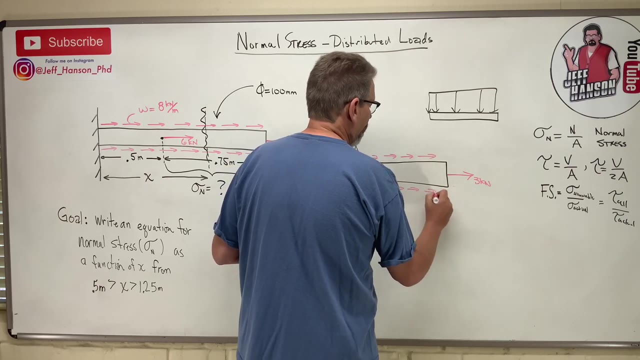 So there's our beam. Now let's put the loads on here with my red pen. I've got a three over here And I've got these distributed loads here, okay, All right. So we need to know a couple of things here. 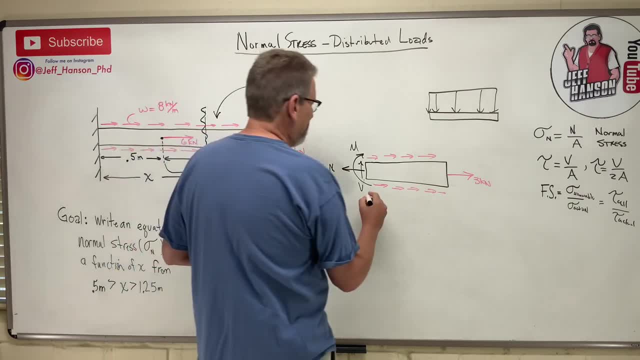 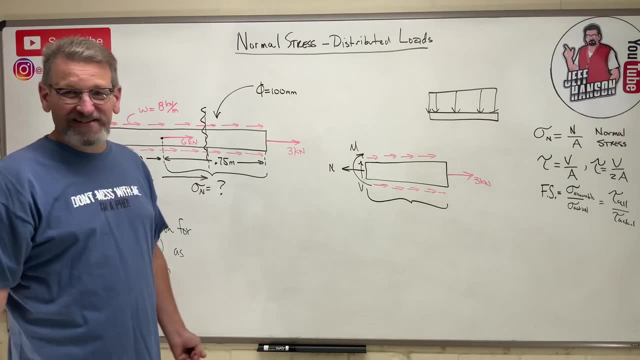 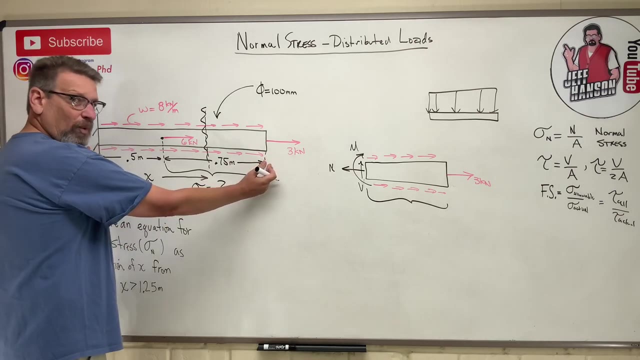 Number one: how long is this beam? How long is that? It's x. No, it's not x, right, x is from the start to there. Well, the whole beam is 1.25, 1.25 meters. 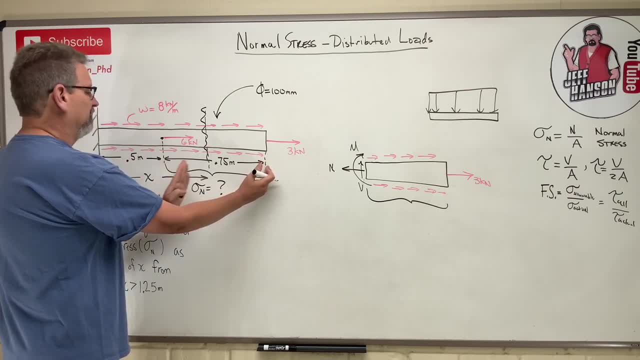 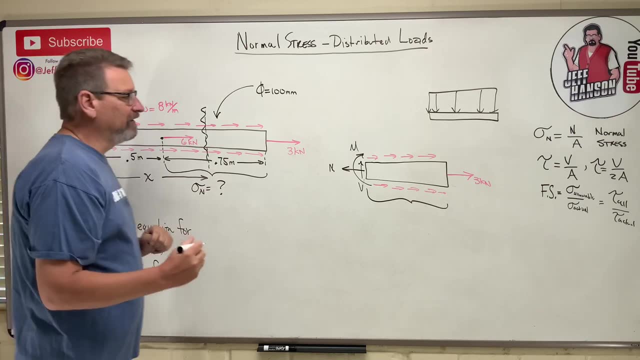 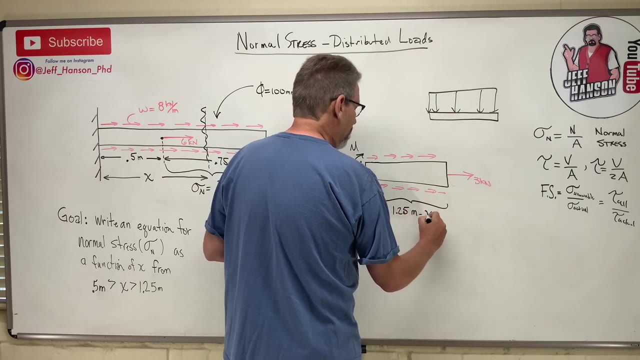 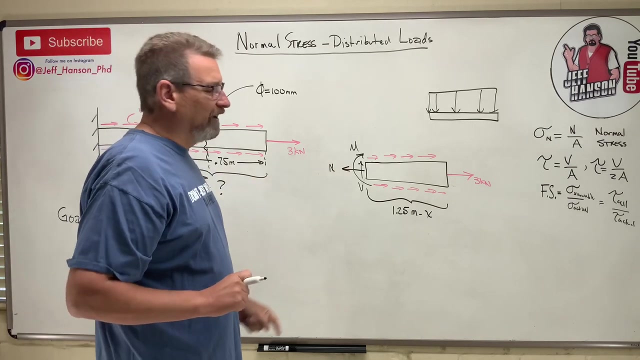 So how far is just that that distance there? The whole thing minus x, right? So this length here is 1.25 meters minus x. okay, So how do we find n? Well, that's, That's not too bad, is it? 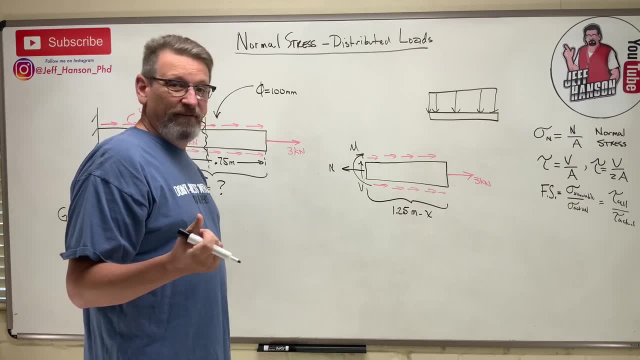 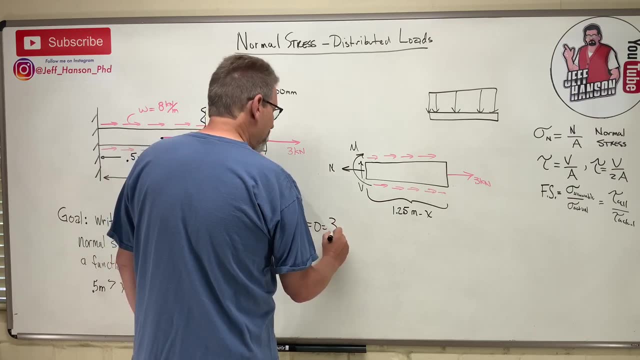 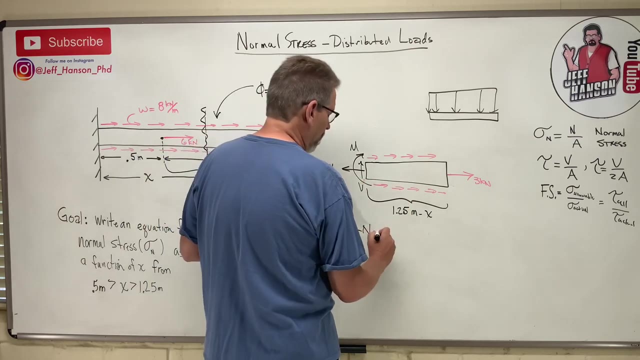 It's just, oh, I don't know, some of the force in the x right, Some of the forces in the x equals 3 kilonewtons minus n, And then also the distributed load. So plus what is the distributed load? 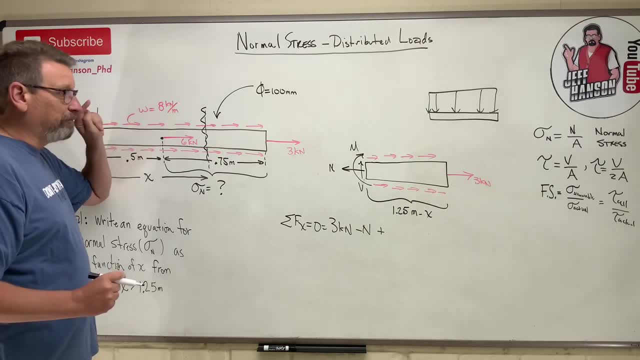 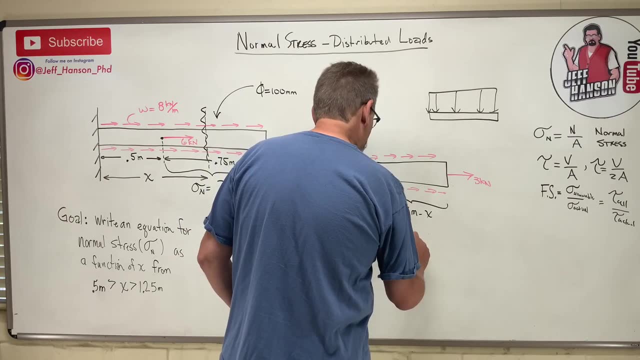 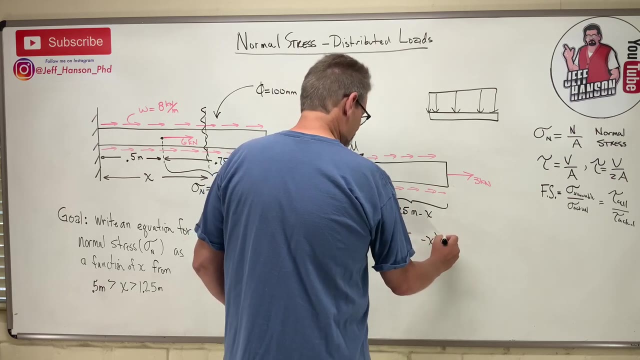 Well, it's 8 kilonewton per meter times how many meters Times that many meters, right? So So 1.25 meters minus x, we'll just say 1.25 times x. we know that's meters times 8 kilonewtons. 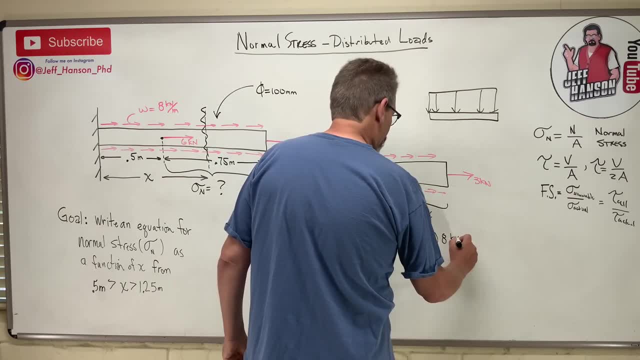 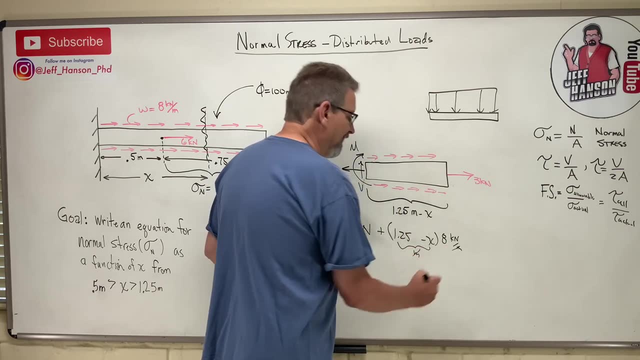 per meter. okay, So if this whole thing is in meters and I multiply that times that, then that and that cancel out. So that's in kilonewtons, that's in kilonewtons. so when I solve for n, it's going to be in. 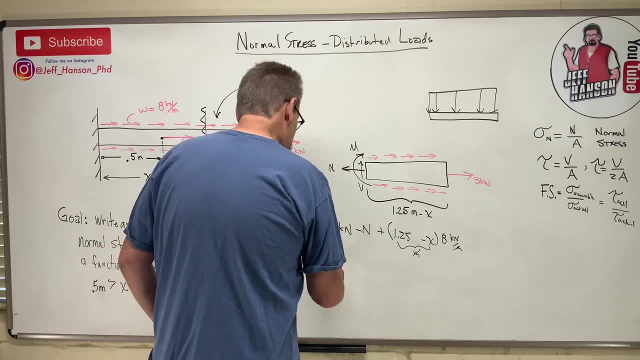 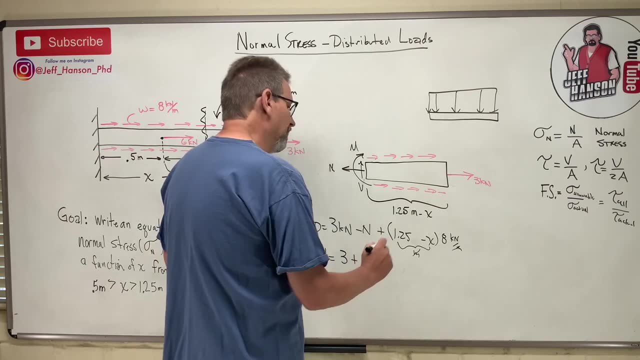 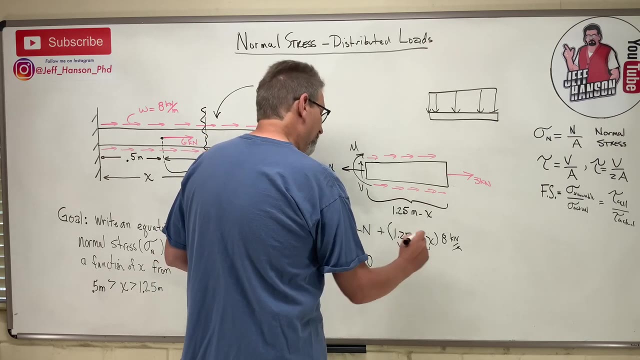 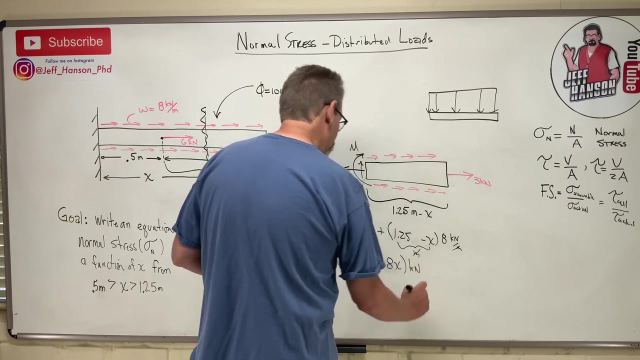 kilonewtons. So move the n to the other side. n is equal to 3 plus 8 times 1.25,. a quarter of 8 is 2, so that's 10, minus 8x, and that whole thing is kilonewtons, right. 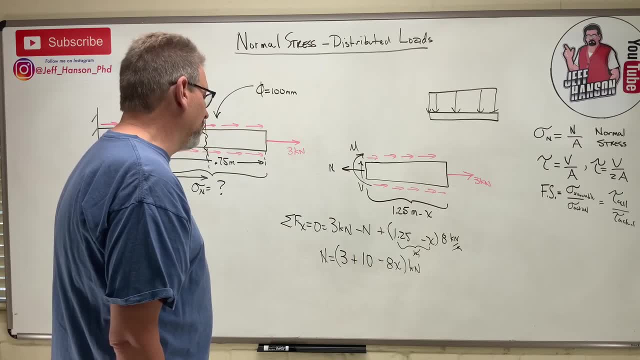 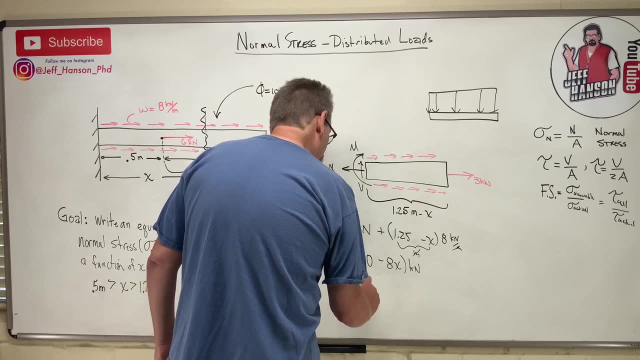 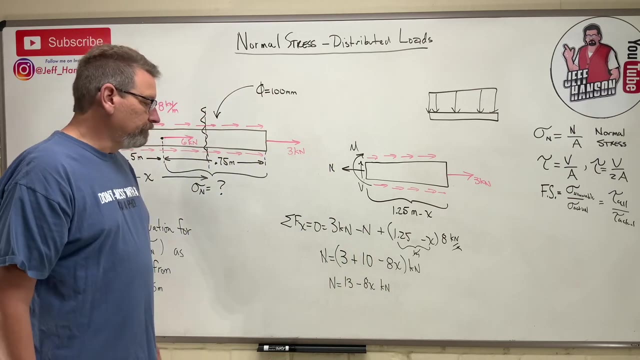 And so let's see: 3 plus 10 is 13.. 10 is equal to 13 minus 8x kilonewtons. okay, Cool, So far, so good. Now they want an equation for sigma n. 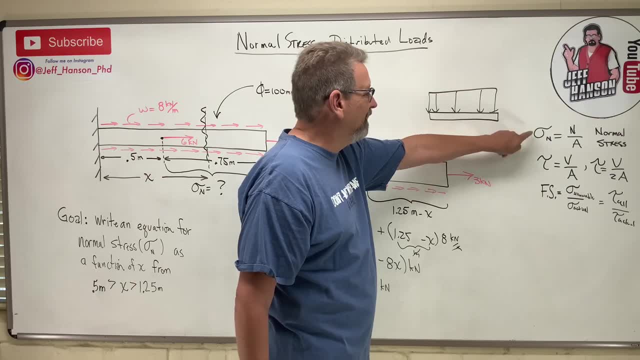 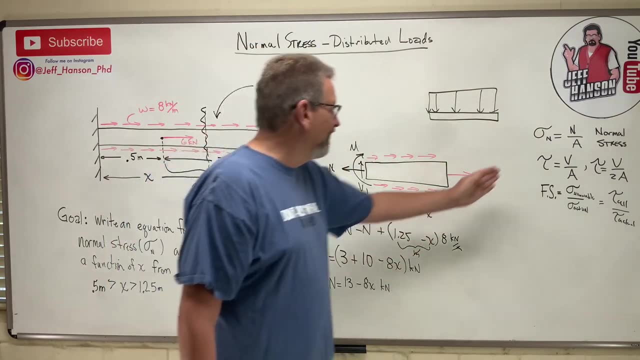 We know. well, we know that, don't we? It's right there, okay, So we're going to use that equation Now. do we know the area? We know n? there's n right there. bam, what is a? 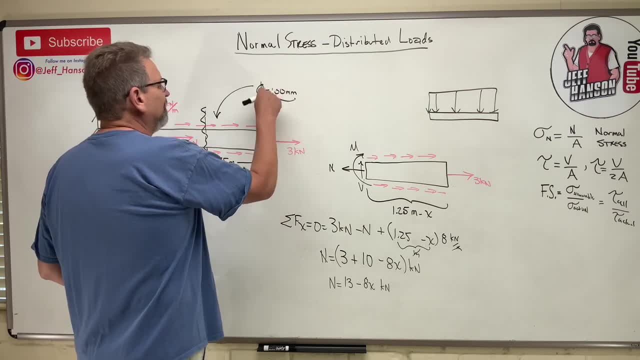 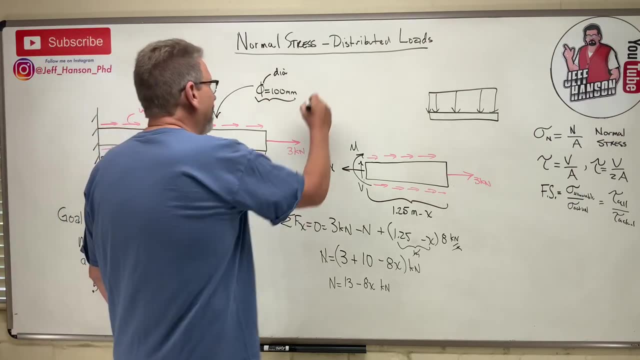 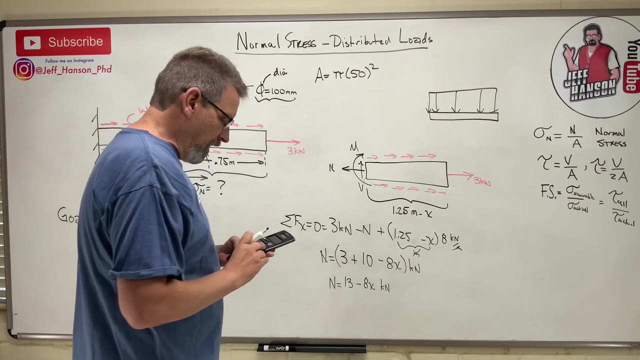 Well, that's pretty easy too. They tell us that this phi, that's the international symbol for diameter, okay, is 100 millimeters, and so a is equal to pi times 50 squared. How much is that? I don't know. 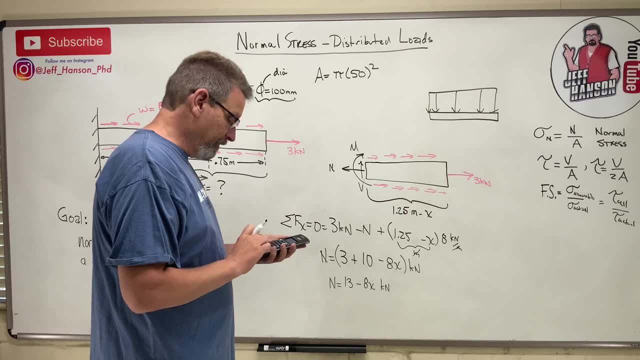 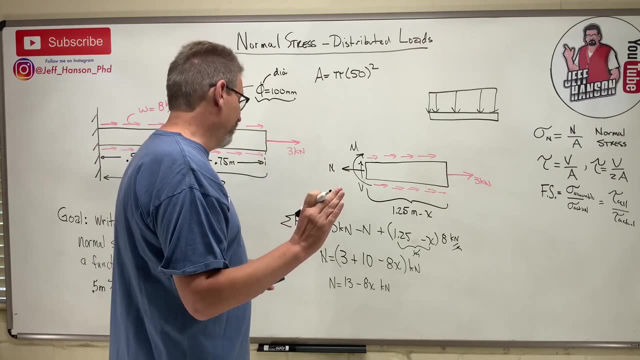 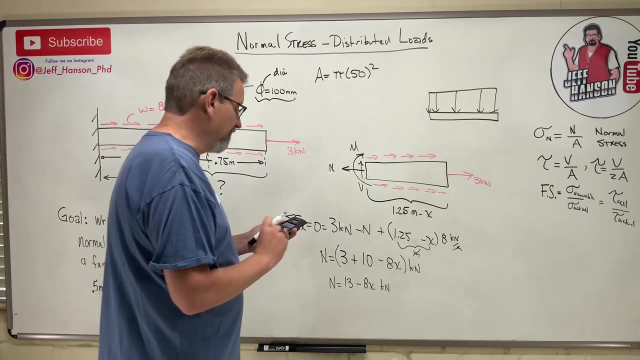 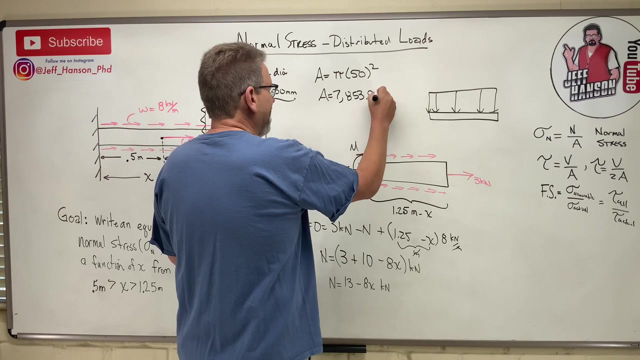 Here we go: Pi par times 50, you know what? Ooh, I don't, let's make sure. Oh yeah, that's okay. Millimeters is good. 50 squared, that's good, And that is: 7,000a is equal to 7,853.98 millimeters squared. 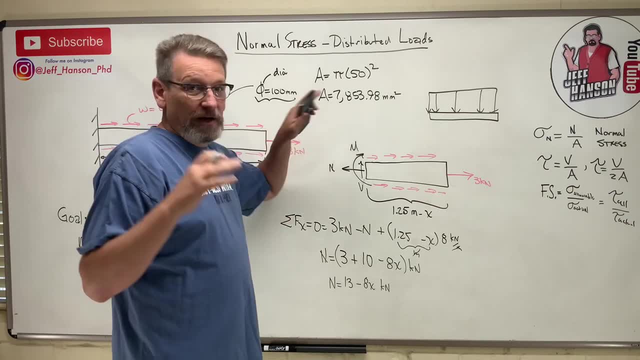 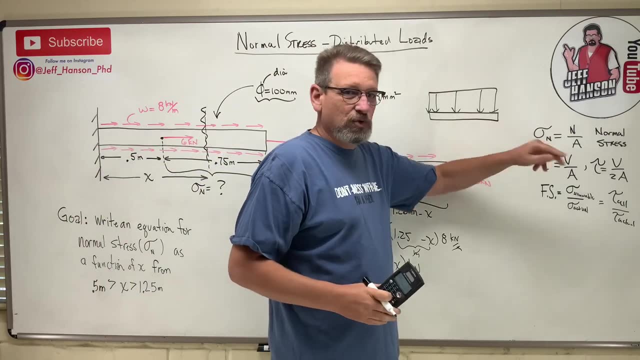 I like that. I'm just going to leave it in millimeters, right? Some of you might be like: oh, it changes to meters. I'm going to change this one instead to newtons. That way I've got newtons over millimeters squared, which is: 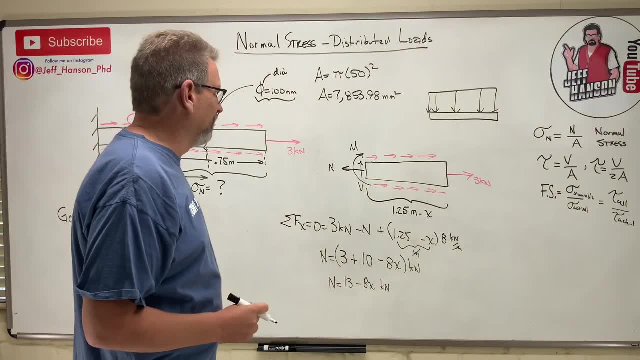 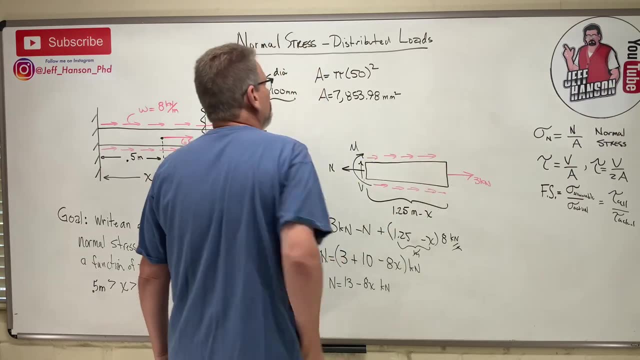 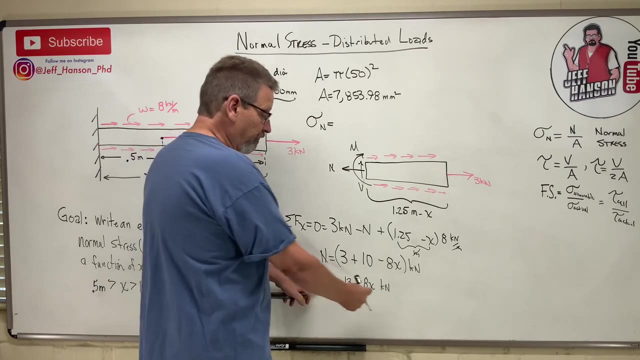 Megapascals way to go. You remembered. Okay, here we go. So let's see here, Let's get rid of that guy. Get rid of that, Okay. so here we go. Sigma n is equal to n, which I'm going to change from kilonewtons to newtons. 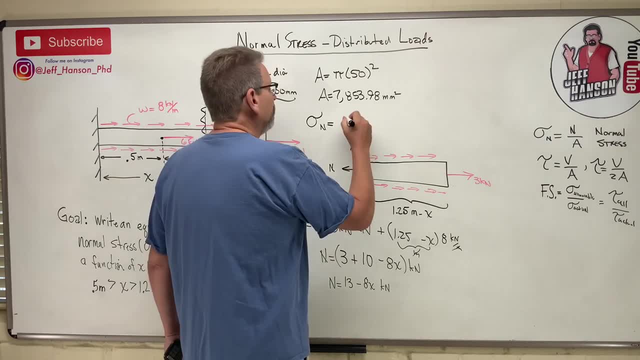 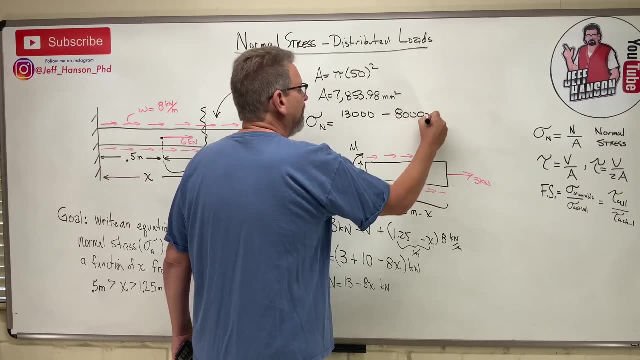 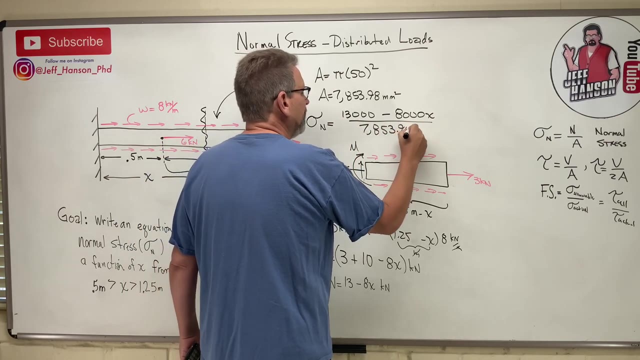 So I'm going to multiply that whole thing by 1,000.. So 13,000 minus 8,000x Divided by the area 7,853.98 millimeters squared. This top is in newtons. 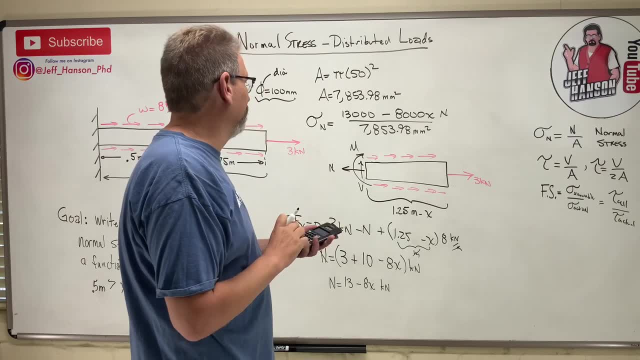 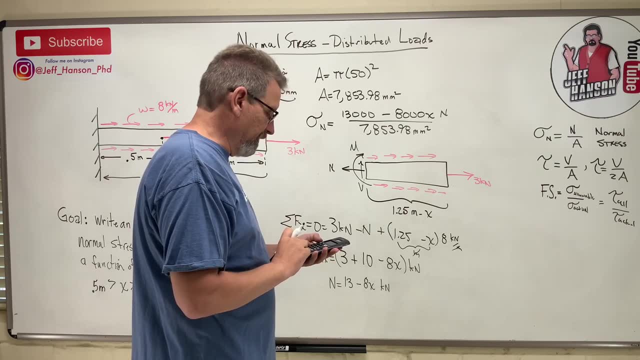 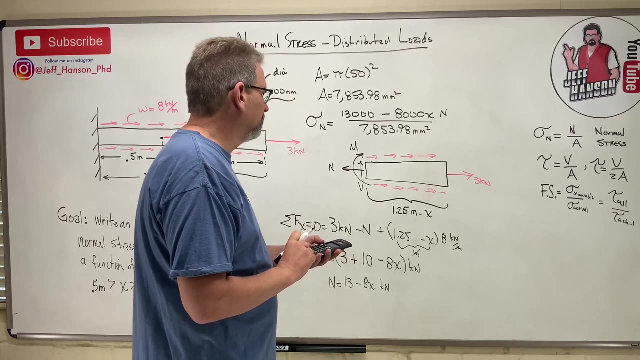 That's going to give me megapascals, isn't it? So 13,000 divided by 7,853.. Minus 8,000.. 8,000 divided by 8,000 divided by. oh, let's just do that. 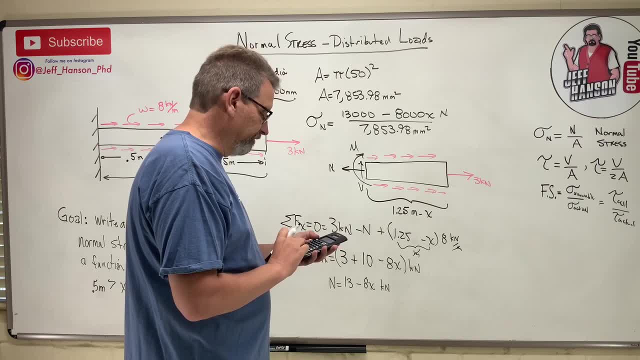 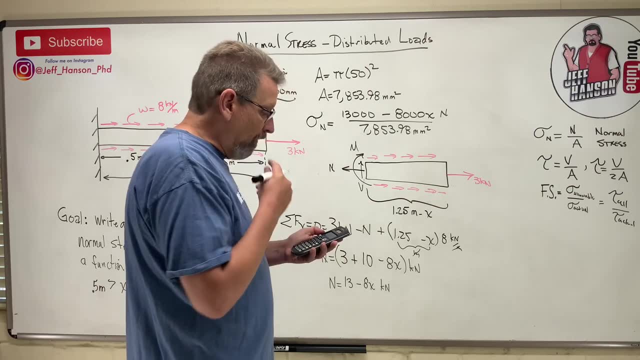 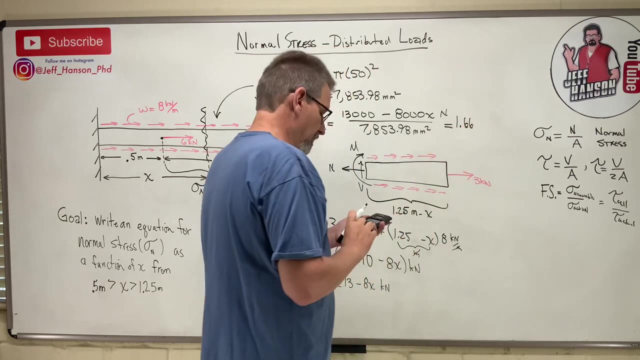 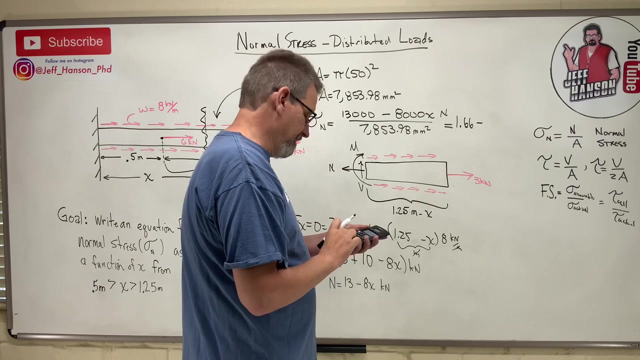 Wait a minute, Let's just do that: 13,000 divided by 7,853.98.. 7,853.98 equals 1.66.. So this is going to equal 1.66 minus 8,000 divided by 7,853.98..